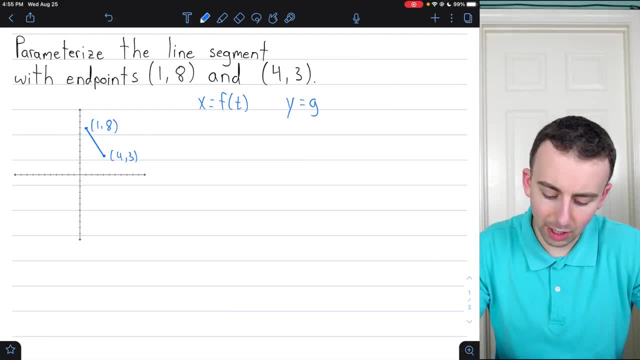 y will be some function of the parameter t. We could say that y equals g of t. And now, since we know the starting point of the line segment and the ending point of the line segment, we know some information about these functions that we're trying to figure out. I'll remind you. 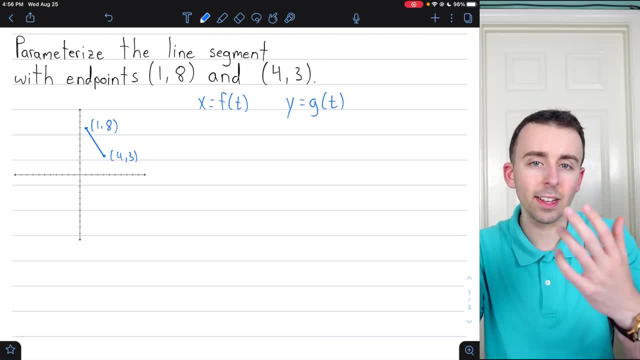 before we get into finding the functions, that parameterizing a curve gives us a sense of direction. In this case, we can assume the segment starts at 1, 8 and ends at 4, 3.. So if this represented the motion of a particle, as t increases, the particle is: 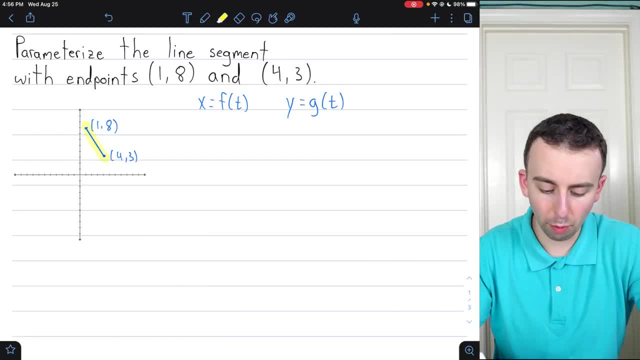 moving from 1, 8 to 4, 3.. So we could just draw an arrow on this line segment indicating the direction. Since this line segment starts at 1, 8 and ends at 4, 3,, we'll want our parameter. 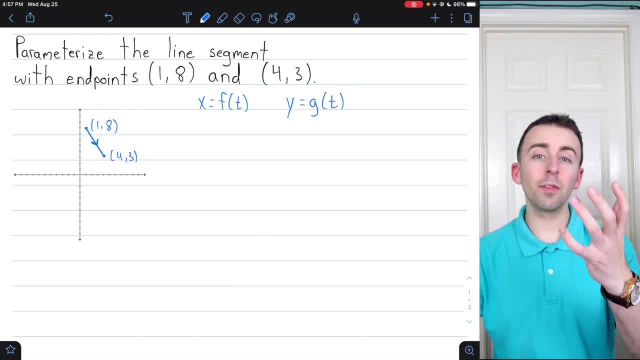 t to be bounded below and bounded above to have some starting point and some ending point. It's not gonna of veer off to infinity or negative infinity. So a very convenient pair of values to bound t with are 0 and 1.. They're really nice to work with. So we could say our parameter t is greater than. 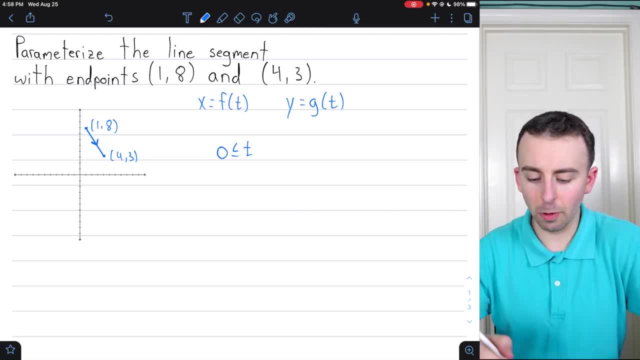 or equal to 0. This means at t equals 0,. the initial point is 1,, 8.. And we'll say that t is less than or equal to 1.. So the terminal point, the final point, is: at t equals 1, where x equals. 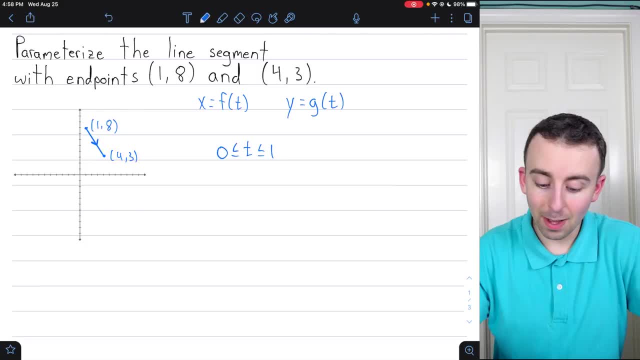 4 and y equals 3.. But there are infinitely many parameterizations we could come up with for this curve, partly just depending on the values we select for t. We could have chosen different numbers instead of 0 and 1 if we wanted to, which would lead to different parametric. 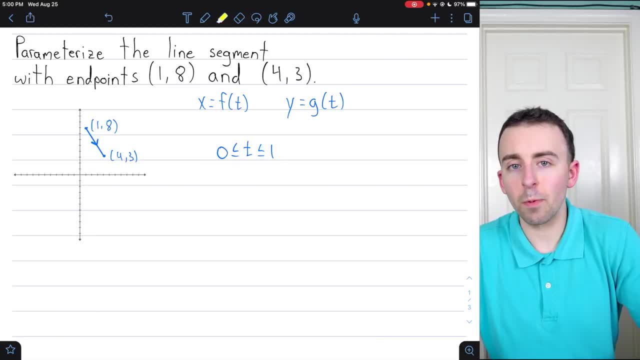 equations, We can often think of a parameter as a number, and we can often think of a number as a number. We can often think of the parameter as representing time. So in that case we can imagine this particle takes 1 second to move from the point 1, 8 to the point 4, 3, where t equals 1.. Whereas 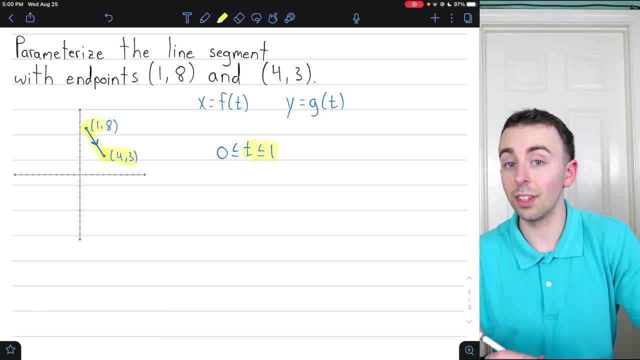 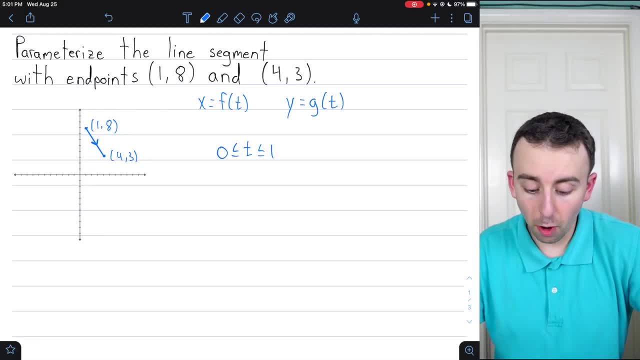 But what is that function? Well, the starting point for x is x equals 1.. So we might just start off by writing x equals 1.. But we know x has to change as t changes. So in order to account for that, 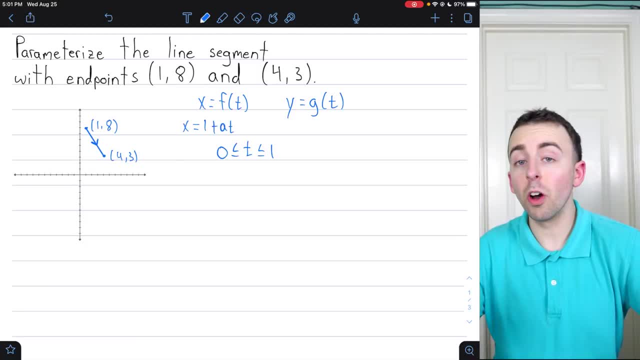 perhaps we add a times t. We don't know what a has to be, but we know there needs to be some term that will allow x to change as t changes. We'll worry about what a is in a minute. Let's do the same thing with y. The starting value for y is: y equals 8.. That's at the initial. 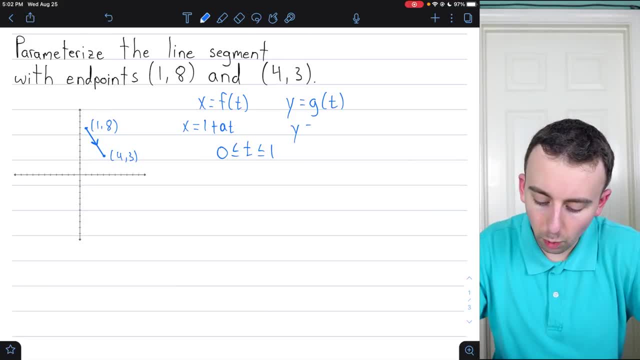 point where t equals 0. So we could write y equals 8.. And again y is going to change as t changes. So we might want to add a term bt. This gives y a way to change as t changes Again. 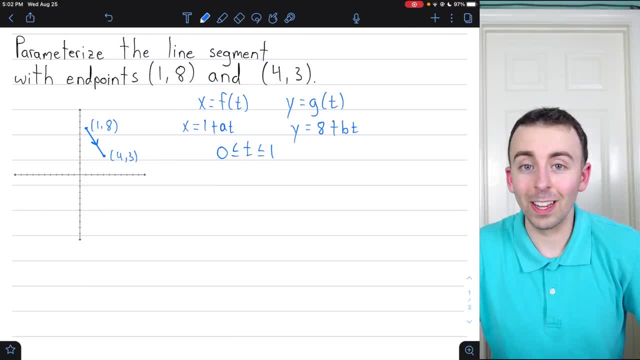 we don't know what b is yet, but we will figure it out. Figuring out what a and b have to be is made very easy by the fact that we chose t to range from 0 to 1.. We can already see that our parametric equations work when t equals 0.. When t equals 0, this plus at will be 0.. And 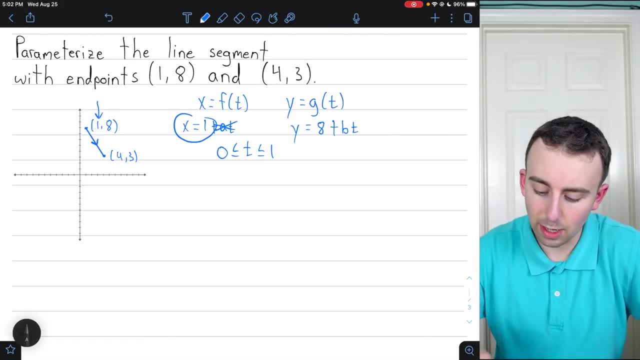 so x equals 1, just like we want. And when t equals 0,, this b times t term will be 0. And so we just have y equals 8, like we want. So we see, when t equals 0,, our parametric equations. 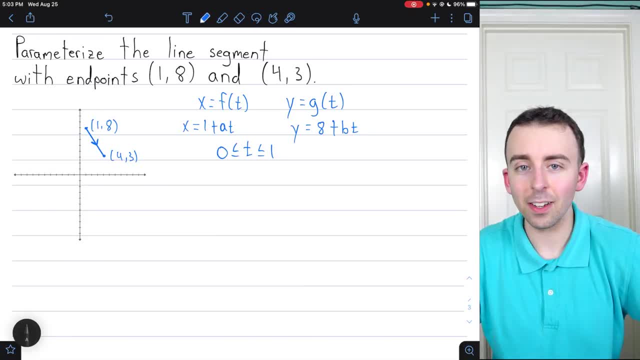 give the correct point of 1, 8.. So now, how are we going to figure out what a and b are? Well, remember, these are parametric equations for a line segment, And what defines a line is that it has a constant slope. So, if we look at the ratio, if we consider two points from a line, 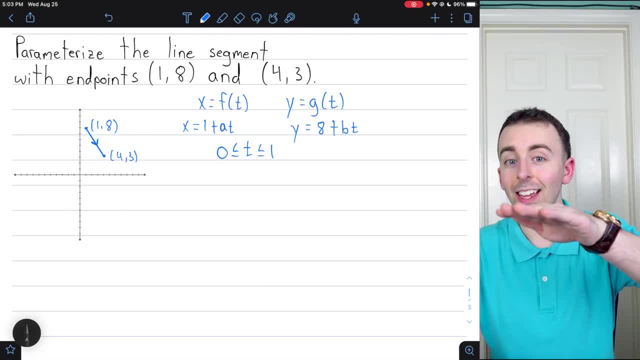 and we look at the ratio of the change in y to the change in x, which is rise over run, which is slope, that should be a constant number. This means, since we already have two points on the segment, namely these two endpoints, if we find the slope between those two points, well, that also has to be the slope. 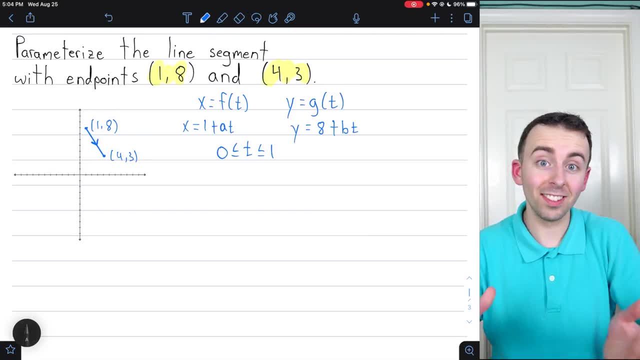 between any other pair of points on the line segment, because it's a line segment And that's what characterizes a line, is that it has a constant slope. And we all know how to find the slope of a line. given two points, We have to just take the second y coordinate minus the first y. 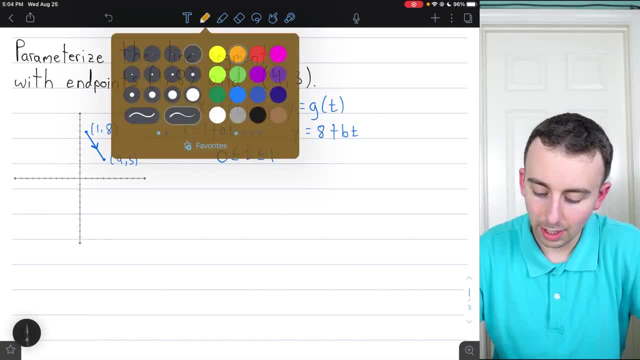 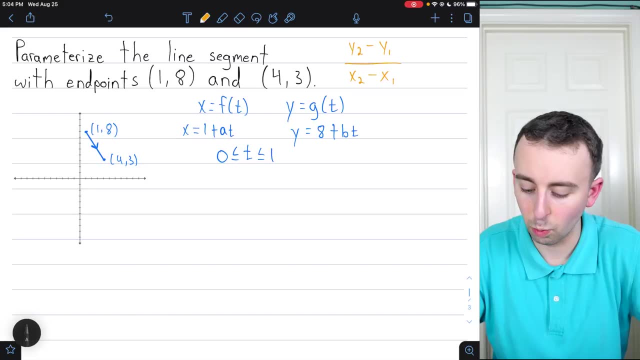 coordinate, So let me just write the formula here in a different color. The slope formula is y2 minus y1 divided by x2 minus x1. It's the change in y over the change in x, In this case the change in. 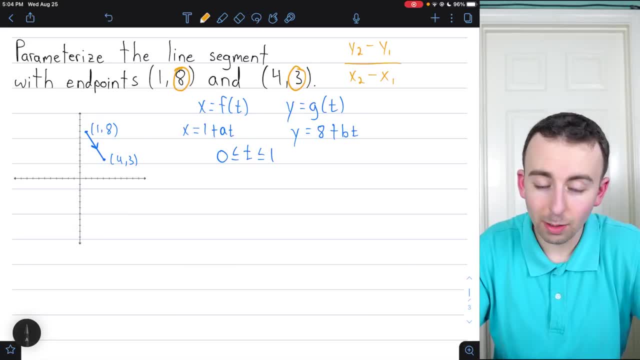 y is what? Well, it goes from y equals 8 to y equals 3.. So the change is 3 minus 8.. And then put that over the change in x. x ends at 4. And starts at 1.. So the change in x is 4 minus 1.. We would also call this the increment in y. 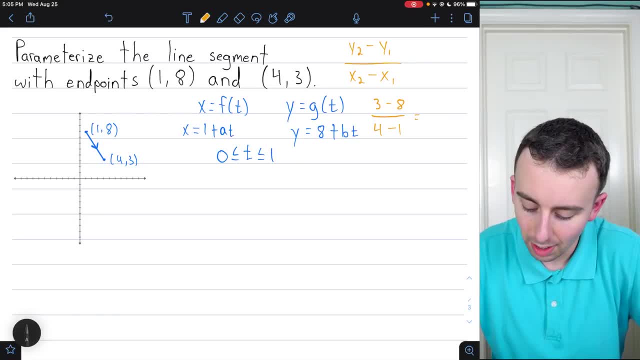 and the increment in x, how much it changed. 3 minus 8 in the numerator is negative 5. And 4 minus 1 in the denominator is positive 3. So what we see is that for every 5 units, y decreases. 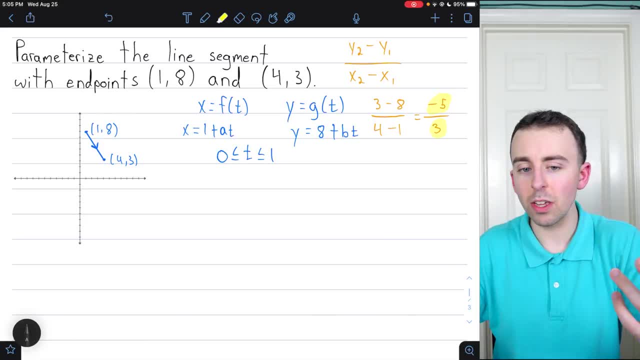 we need x to increase by 3 units. That's how y and x relate. Now, when t equals 1, at this terminal point we will need y to have gone down 5 units from 8 to 3.. That's a decrease in 5. Which means this coefficient b next to t. 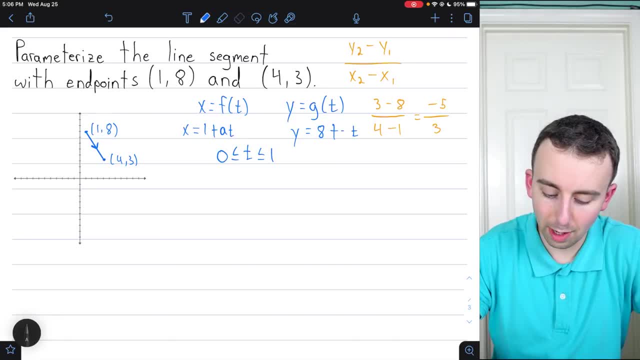 should be negative 5.. So instead of writing plus negative 5, we'll just write minus 5.. So the equation for y is: y equals 5.. And we'll just write minus 5.. So the equation for y is y equals 5.. 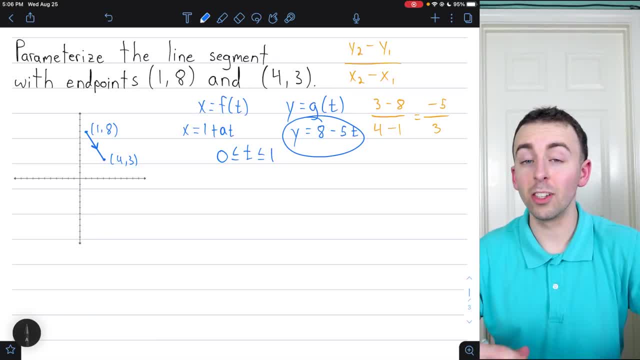 Again, this is because the change in y is a decrease of 5. So minus 5.. Now when we plug t equals 1, the terminal point- into this equation, we'll get 8 minus 5, giving us that y coordinate. 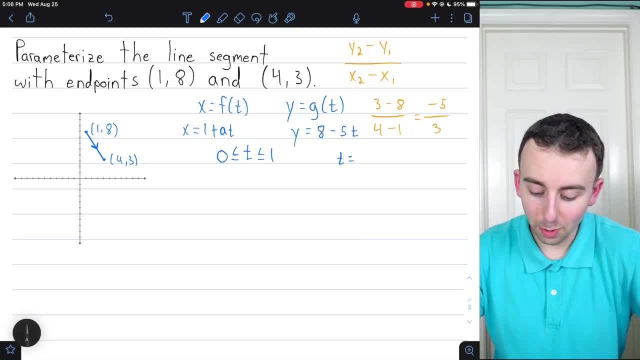 of 3 that we want. Now we also know: if y is going to decrease by 5 units, what does x need to do? Well, we just figured out. the result is negative: 5 over 3.. When y decreases by 5, x needs to go up by 3.. And so this coefficient. 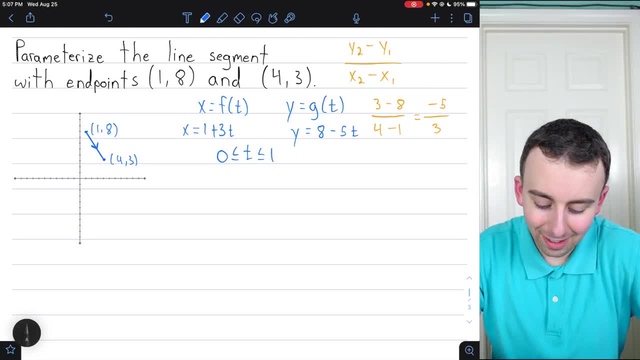 a over here in the equation for x is 3.. The equation for x is 1 plus 3t, And now we have parameterized the line segment. So in these equations if we plug in, t equals 0 to get our initial point, we'll have 1 plus 0 for x, which is 1. And we'll have 8 minus 3.. And we'll have 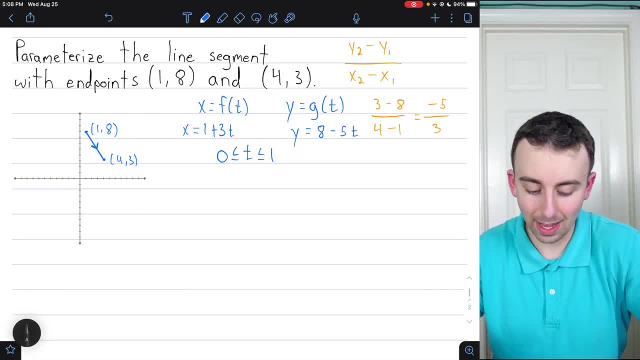 minus 0 for y, which is 8. And that will give us the correct point of 1, 8.. And then for the terminal point, we'd plug in: t equals 1.. That would give us 1 plus 3 for x, which is 4.. And 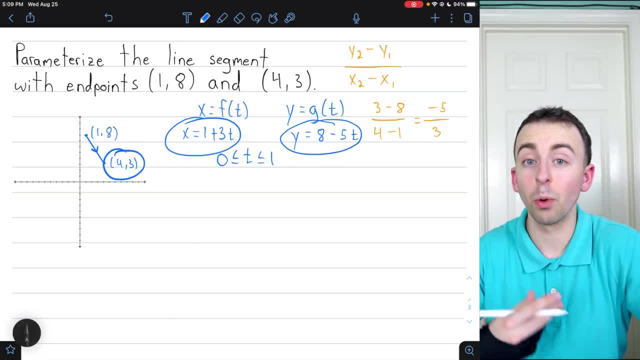 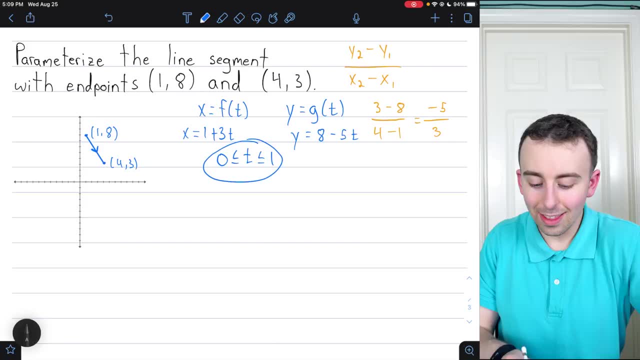 8 minus 5 for y, which is 3.. That point for 3, that's the correct terminal point. Now, if we were to change the bounds on t, these parametric equations would not be correct anymore. They would not produce this line segment If t could go all the way up to 2,, for example. well, in a way, 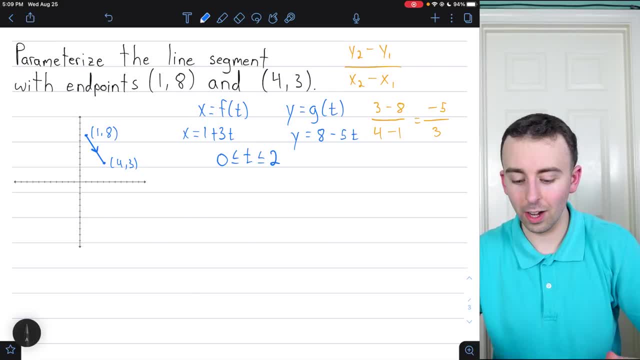 that means that the motion is taking twice as long, which means the change in y is going to have to be half as fast And the change in x will need to be half as fast, which means our new equations. in that situation, we would need 3 over 2 times t and 5 over 2 times t. Again, you can see. 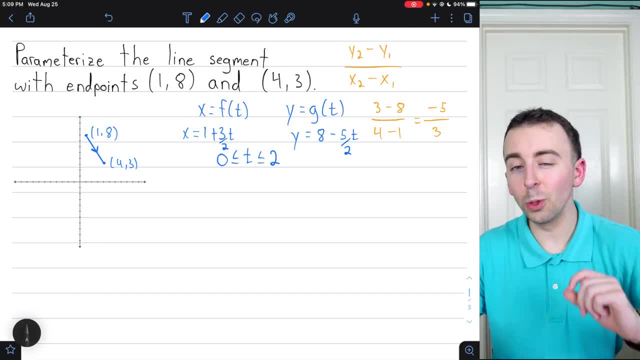 how, if we plug in t equals 0 to get our initial point, we'll have 1 plus 0 for x, which is 5.. And if we plug in t equals 2 to those equations, we'll get the correct terminal point having. 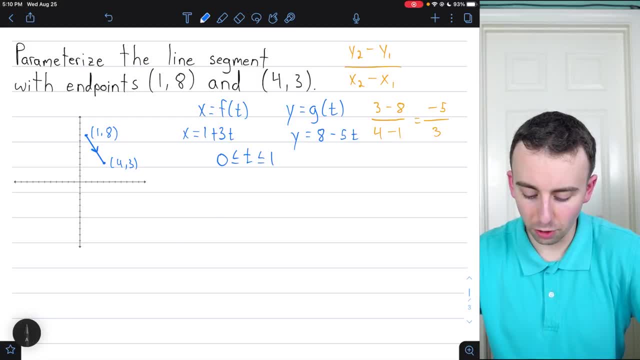 accounted for that change in t value. But let's undo and get back to our original bounds. One last thing you might want to do, just to check: do these parametric equations actually produce a line? We could eliminate the parameter in order to find out. So let's solve for t in terms of x. 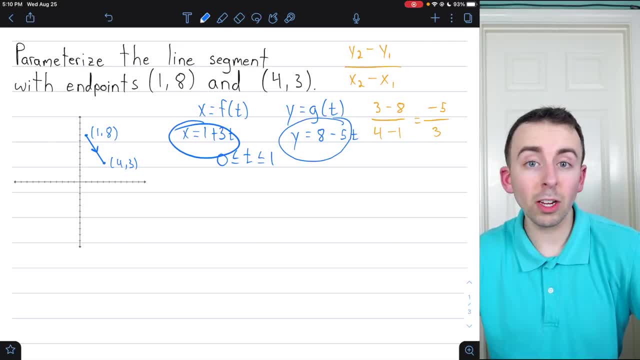 and then substitute that into the equation for y to make sure that we've got a line. So I'll rewrite the equation in green Over here. the parametric equation for x is 1 plus 3t. To solve for t we'll subtract 1 from both sides, So x minus 1 equals 3t, and then divide both sides. 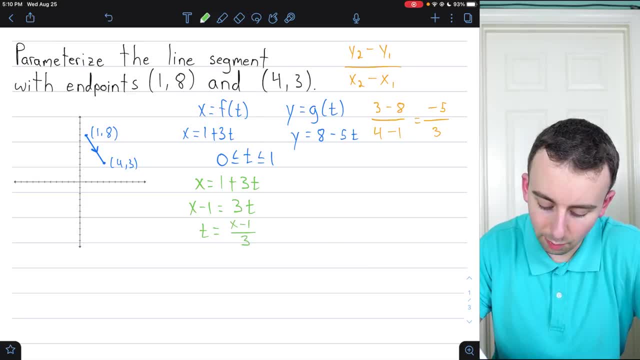 by 3.. So t equals x minus 1 divided by 3.. Now we can substitute that in to the equation for y: y equals 8 minus 5t, but t is x minus 1 over 3.. And now we can actually make this look pretty nice if we subtract 8 from both. 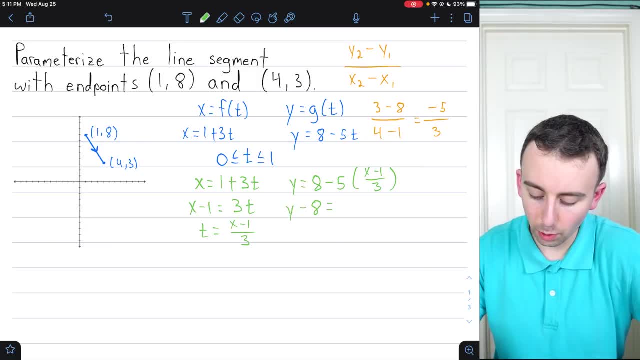 sides. Then we'll have y minus 8 equals. let's take the 1 third out of that- x minus 1.. So this is going to be equal to negative 5 over 3.. We just took the 1 third out of the parentheses. 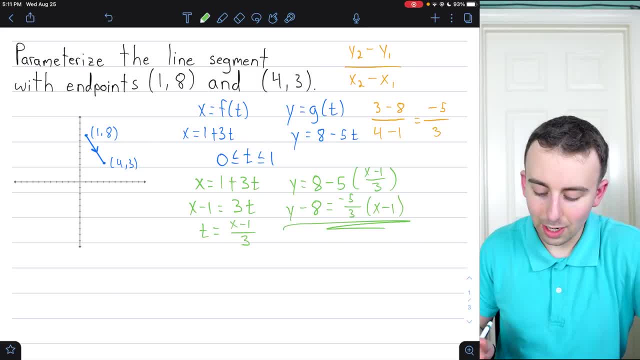 multiplied by x minus 1.. This is clearly the point slope form equation for a line. So we're good, We've got parametric equations that give us this line segment with end points 1, 8, and 4, 3.. So the process here is really simple If you're trying to parameterize a line segment. 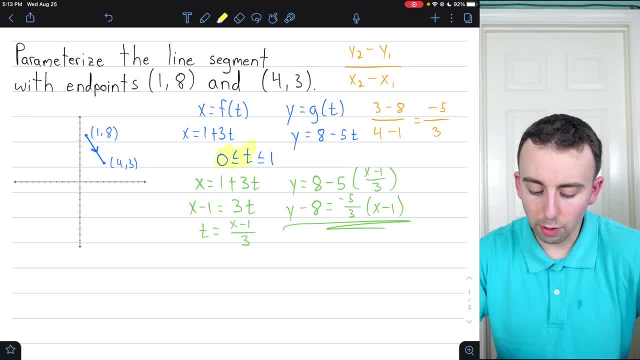 and you're given the end points. you can just let t range from 0 to 1.. Then the parametric equation for x is the initial x coordinate plus the change in x times t. You can see our initial x coordinate is 1, the change in x was going from 1 to 4.. So 4 minus 1, that's a change of 3, that's our. 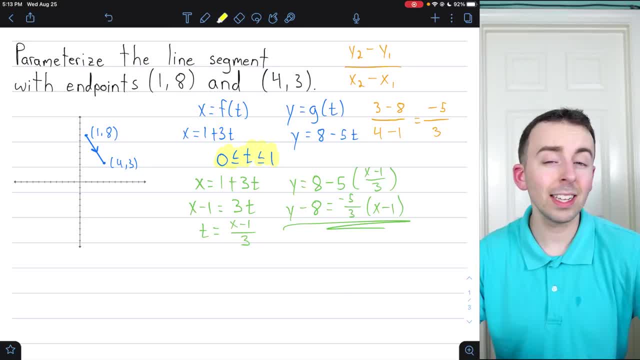 coefficient for t And the parametric equation for y is found in a similar way. y equals the initial y coordinate plus the change in y times t. The change in y was minus 5, so we have minus 5t. I think you'll agree that's pretty straightforward, but let's go ahead and do. 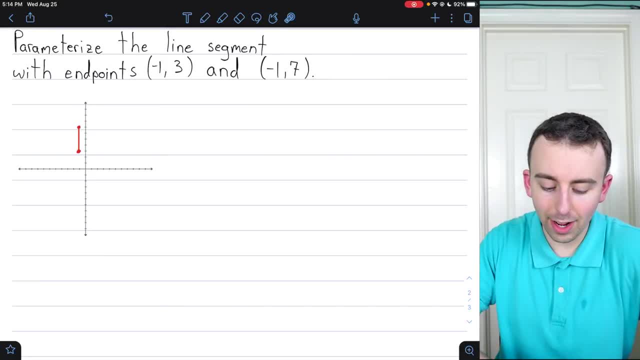 one more example: We're asked to parameterize the line segment with endpoints negative 1, 3 and negative 1, 7.. And here is that line segment there. Since it's going from negative 1, 3 to negative 1, 7, I'll draw an arrow there indicating the direction of the segment. Now we can quickly. 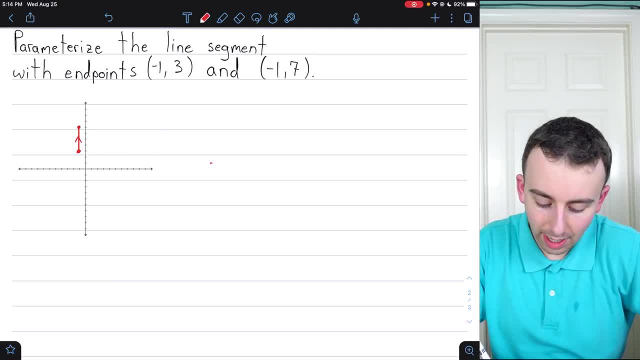 go through the thought process we did last time, We can say that our parameters t is going to range from 0 to 1.. We know that x is going to equal its initial coordinate negative 1, plus something times t, And y is going to equal its initial coordinate of 3. 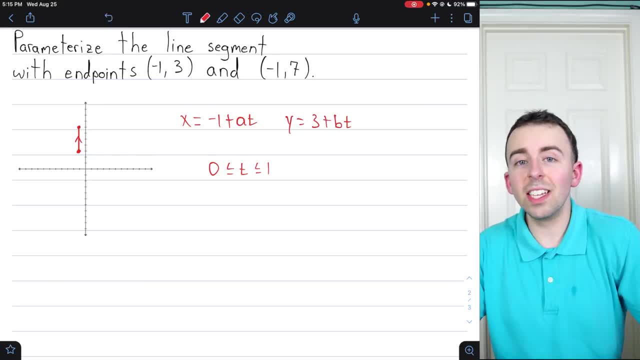 plus something times t. Then we considered the slope of the line. Perhaps you can see that something weird is going to happen here. The slope of this line is going to be the change in y or the rise in y times t, And we're going to draw an arrow there indicating the direction of the 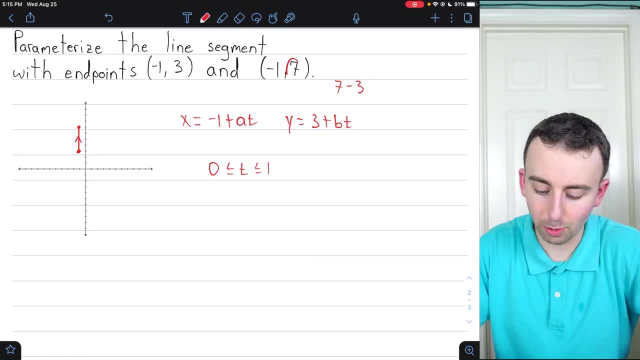 rise, which is 7 minus 3,. right, That's the change in the y coordinates divided by the change in x. Let me move this up a little bit. The change in x is negative: 1 minus negative 1.. Negative: 1 minus. 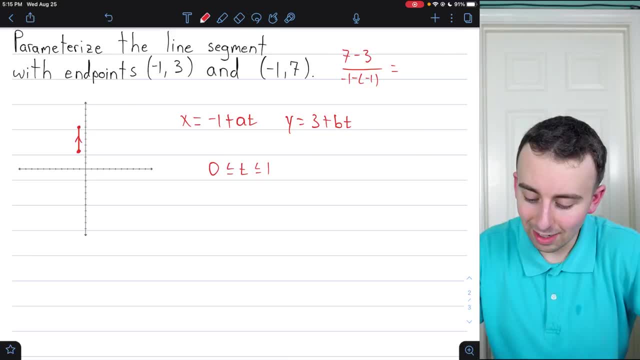 negative 1.. And this: the slope of the line is equal to 4 over 0.. Oh man, that looks bad. right, We can't divide by 0.. That's an undefined slope, But it's still really no. 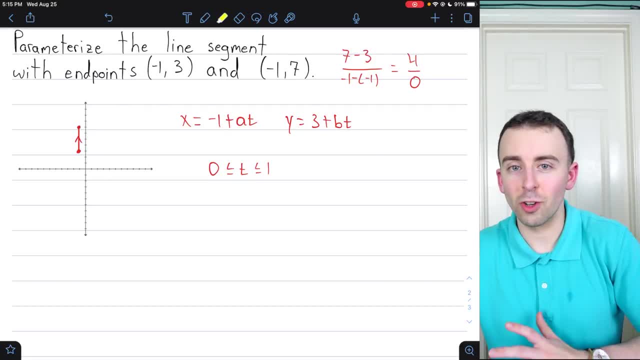 problem here. This is just telling us that x is not changing based on a change in y. When y changed 4 units, how much did x change? Not at all. So this means when t equals 1, we'll need y to have increased by 4 units, because that's how much y changed. So the coefficient of t